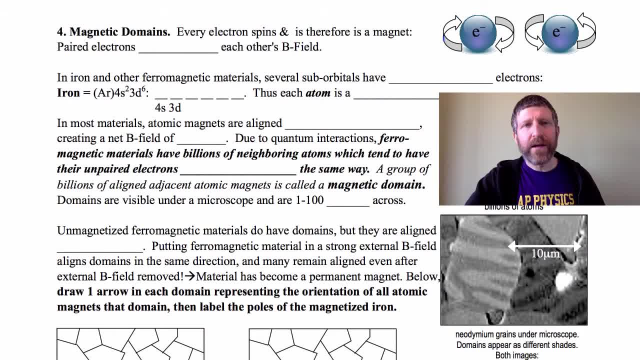 Now we can talk about magnetic domains. Magnetic domains are what make permanent magnets permanent magnets, and without them that we would have no permanent magnets. It's present in all materials which are ferromagnetic. We have to start with understanding that every electron spins. Now, if 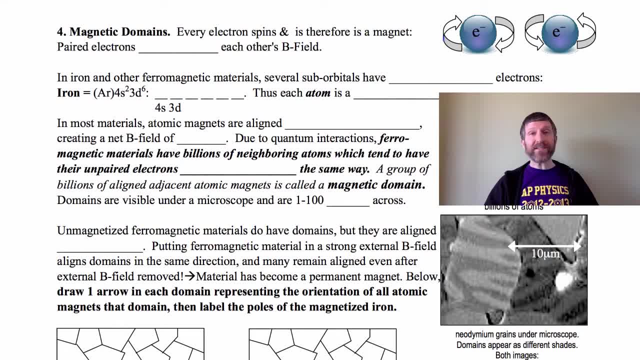 you talk to a quantum mechanic, they'll say, well, it really doesn't spin, but it sure acts like it's spinning. So we can just use this assumption of classical mechanics that the electron is spinning and to figure out what its magnetic field looks like. So let's take a look at this electron first. 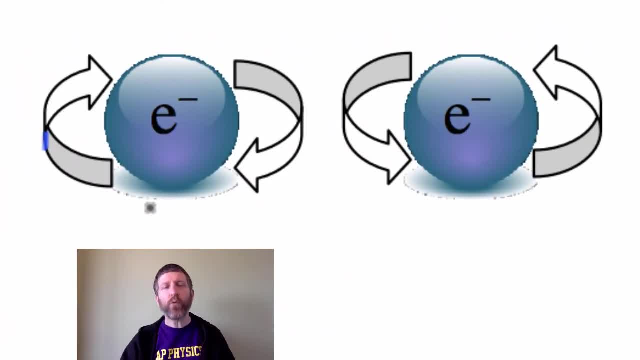 on the left and if you use your coil right hand rule, we can figure out which end of this spinning electron is the north magnetic pole. So you've got to use the left hand rule because it's an electron and you can see that in this situation on your left it's curling into the page. It's like a spinning electron this way. 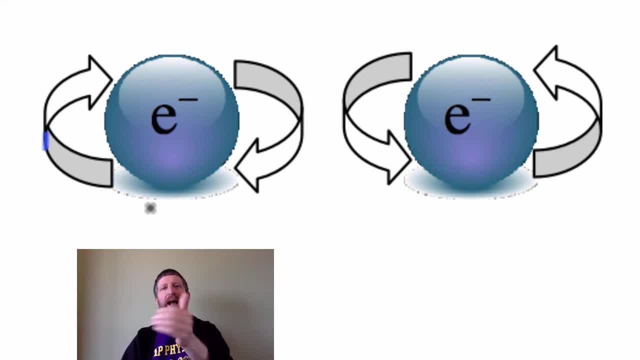 it's spinning, use the left hand rule and on your right it's going out of the page. So by curling your fingers around like this in the direction of the spinning electron, you can see that the north pole of this electron is towards the top and the south pole is towards the bottom. The other 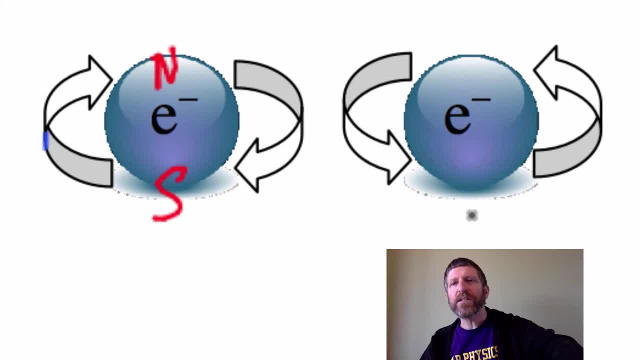 electron, this one on the right, by contrast, that is spinning the other way: On your left it's going out of the page and on the right it's going into the page, So that using the left hand rule is pointing down Again, we use the left hand rule. 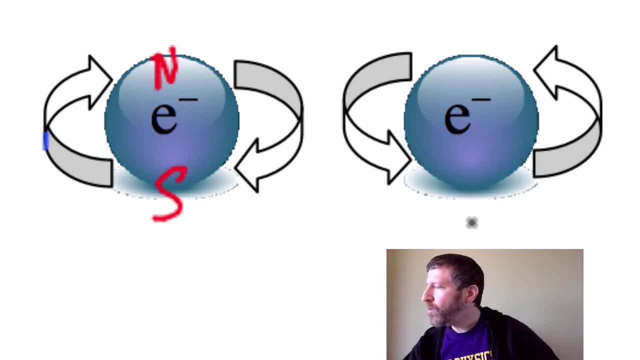 because it's a negative charge spinning around, So that'll give us the north pole down and the south pole up. If you draw your magnetic field lines in like this, it comes out of the north end but then immediately goes into the south end of this. one comes back out there and curls back. 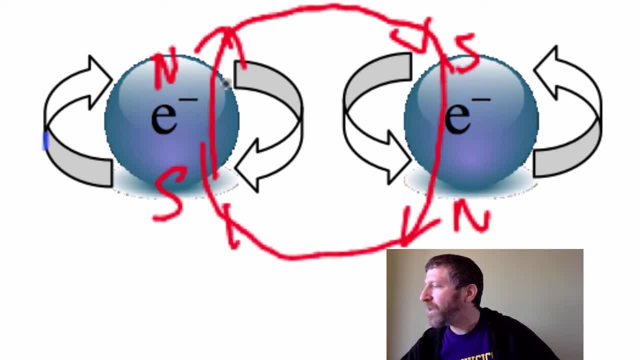 around. So it's forming a closed loop that's like this, which effectively cancels each other's B field. It keeps the magnetic field lines in really tight loop right there. If you have paired electrons, you don't really have a strong B field, You have basically nothing. 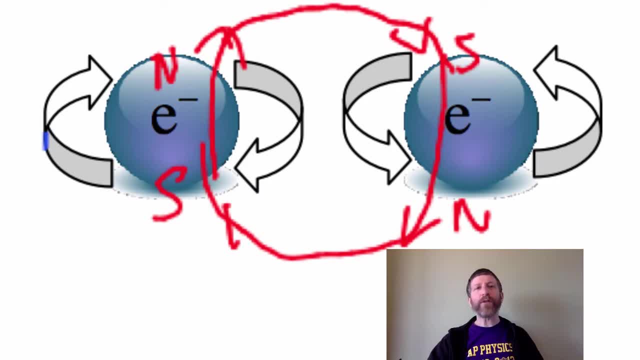 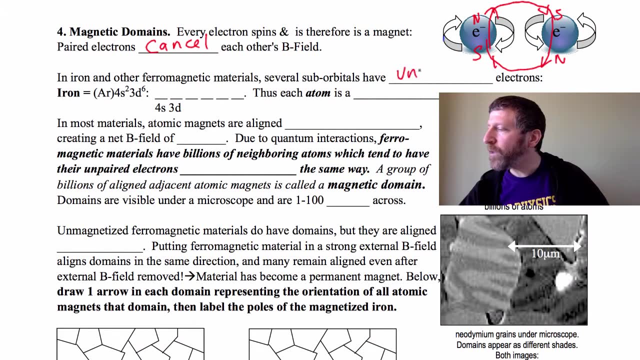 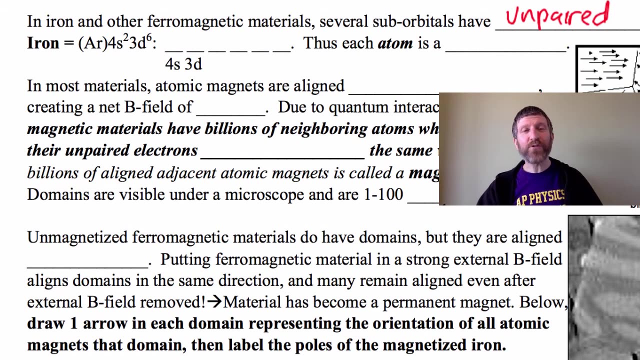 because they cancel each other's B field. However, in iron and other ferromagnetic materials, several sub orbitals have unpaired electrons. Here's an example. Now, you may have done this in chemistry, where you do these little up and down arrows, What you were actually drawing, although 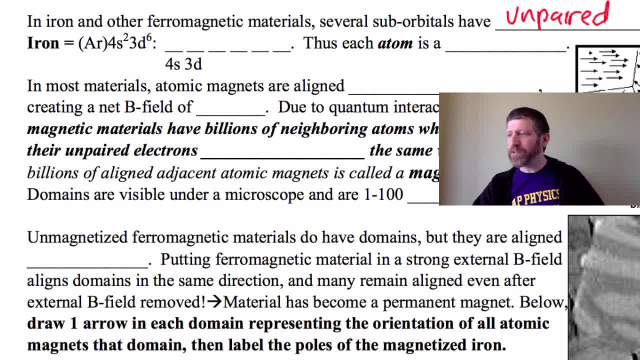 you're not sure. what you were doing was the magnetic polarity of those electrons. For example, in iron we have an argon core, but then we add 4s2 and 3d6. So that means that all you got to do is you first fill in. 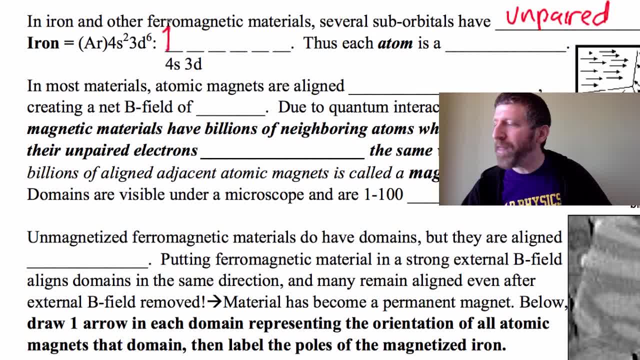 the 4s shell spin up the north pole, that electronic magnet is pointed up and spin down. so we fill those in first. Then we start filling in the 3d orbital with ups: Spin up, north pole, up, north pole, up, north pole up. 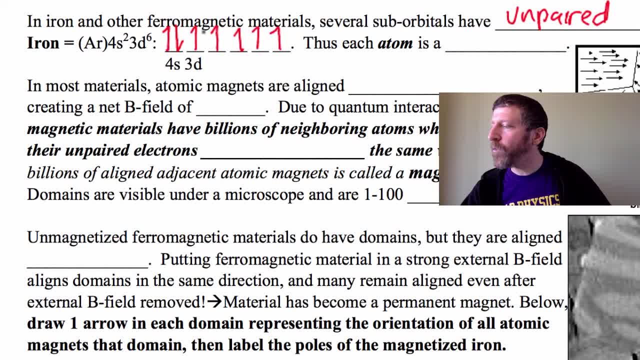 4 and 5.. But then we have another one that we have to do. spin down right there. So you will notice that several of these electrons are unpaired. All these right over there have no pair. So every atom is a magnet. Every single atom of iron is a magnet. Now any 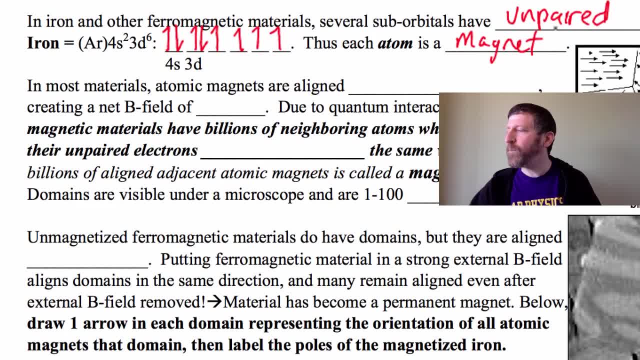 any material that's got unpaired electrons exhibits what's called paramagnetism, which is a weak magnetic effect, But certain things like iron, nickel and cobalt have ferromagnetism, which is an even more powerful magnetism. It has to do with what we're talking about now: domains. 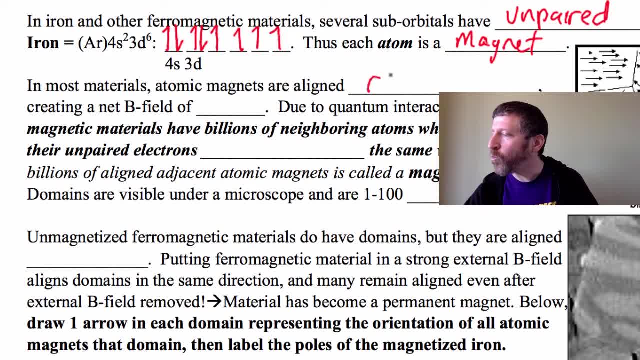 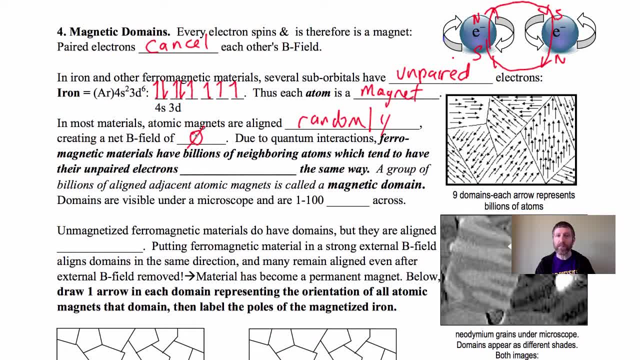 Now, due to quantum mechanics, there are a lot of things that can be done to make a magnet. Some materials- nickel, iron and cobalt to be specific- are ferromagnetic materials, and what they have is billions of neighboring atoms which tend to have their unpaired electrons. 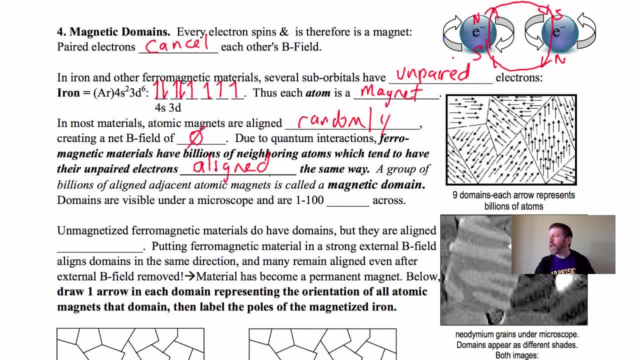 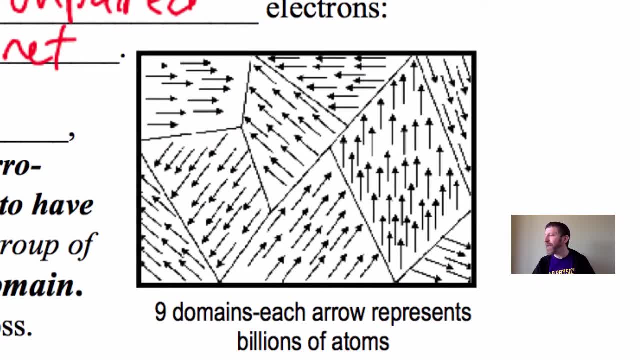 aligned in the same direction. A group of billions of aligned adjacent atoms- that are atomic magnets is called a magnetic domain and in this picture right here, every one of these sections here is a magnetic domain. Each one of these sections has billions of aligned atomic magnets. I'm 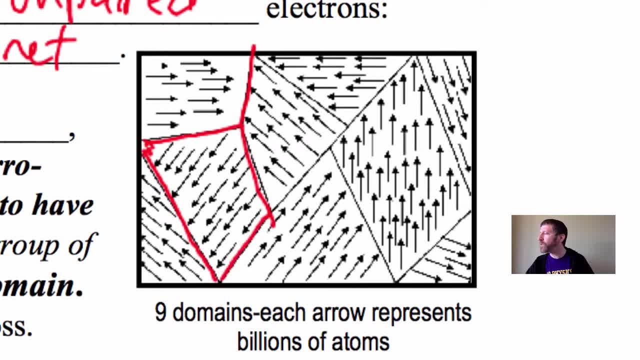 outlining the domains. Now, each one of these arrows, each one of these individual arrows, like this one and this one and that one, those each represent billions of atoms. So we're talking about many billions of atoms. This drawing right here has nine different domains, and each arrow in that 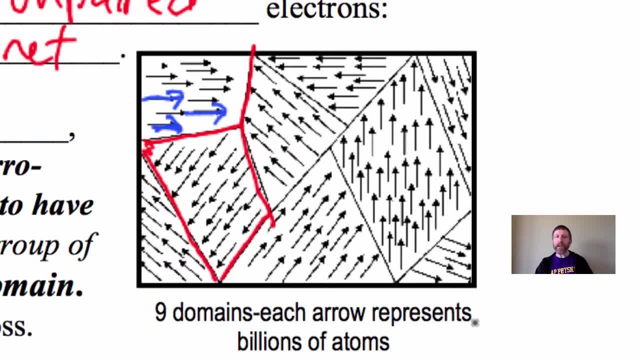 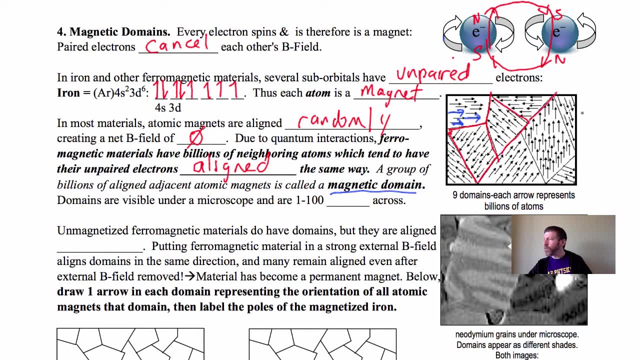 domain represents billions of atoms. So a group of billions of atoms is called a magnetic domain. Now, the group of billions of atoms that are aligned magnetically- they are aligned adjacent atomic magnets- is called a magnetic domain. So here's another domain, here's another domain. 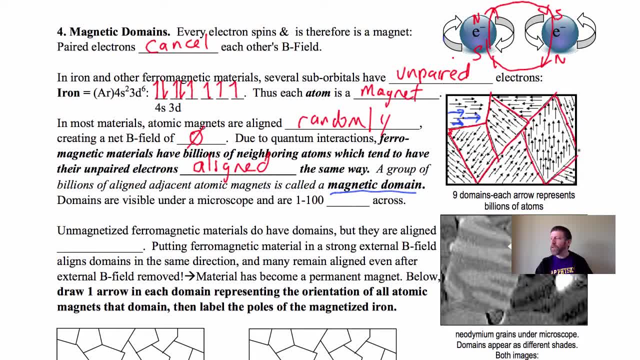 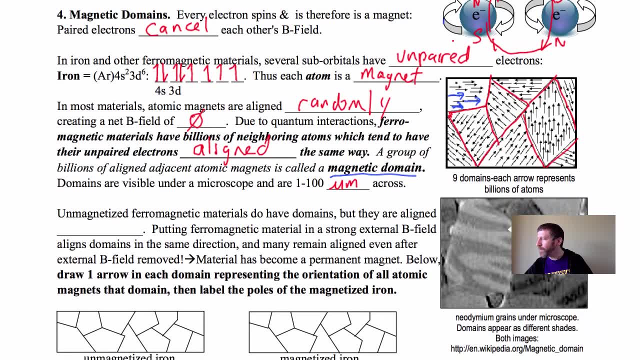 here's another domain, So you can see these domains. Now these are visible under a microscope. They're typically like one to a hundred micrometers across. Here's a picture right here. This right here is an actual picture. What you see as a different? 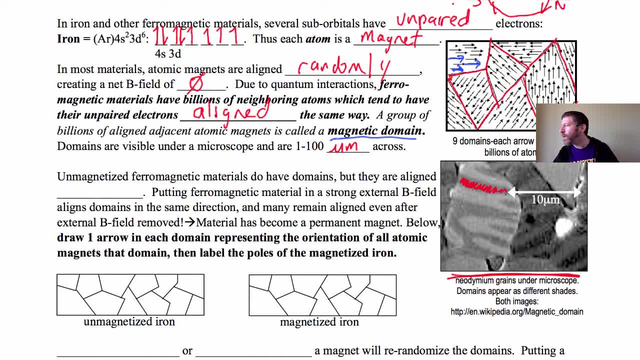 color right in there. that is all one domain right in there And you have another domain right here and it's kind of shaped like that: Here's another domain right there, Anywhere you see a different color. that's a domain, a section of atomic magnets that are 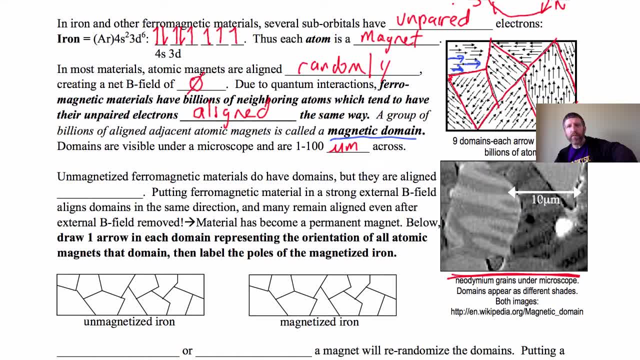 all aligned the same way. So that's what we're looking at right there, And this length right there is 10 micrometers, so you can see how big the domains are: Unmagnetized ferromagnetic materials. but the domains are aligned randomly. In other words, let's draw a picture of this, For example: 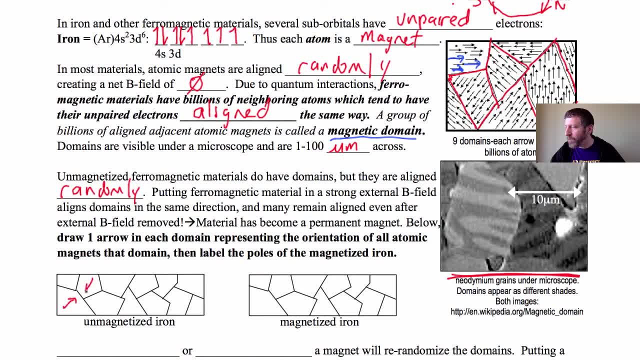 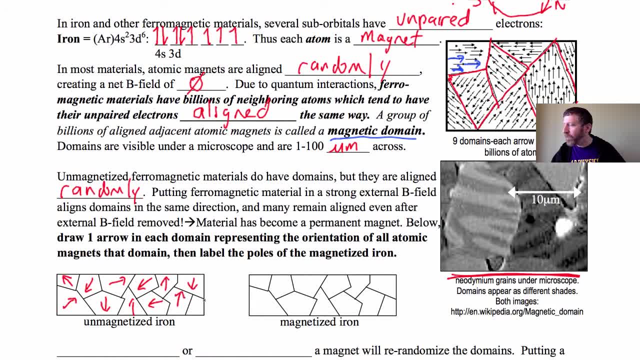 every domain with one arrow showing how the billions of magnets, or atomic magnets, are aligned Here. in this picture up here, every arrow represents billions of atoms. In this picture right here, every arrow represents a single domain with its atomic magnets aligned in the direction. 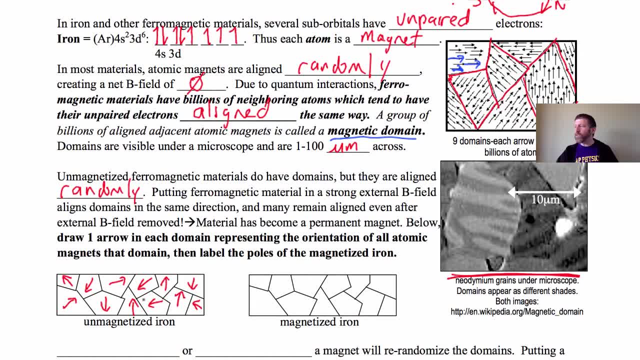 shown here. So what you do is, if you put a ferromagnetic material in a strong external B field, it aligns the domains in the same direction and many will remain aligned even after the external B field is removed. Here's a really cool applet that shows exactly that. So what we have here is a ferromagnetic 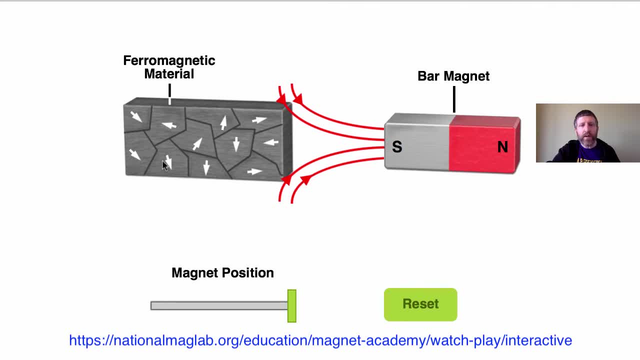 material and this represents the alignment or the orientation of each of the domains. Notice, they're aligned very randomly. What I'm going to do is I'm going to take this bar magnet which will provide an external magnetic field to this ferromagnetic material. I'm going to move the bar magnet close. 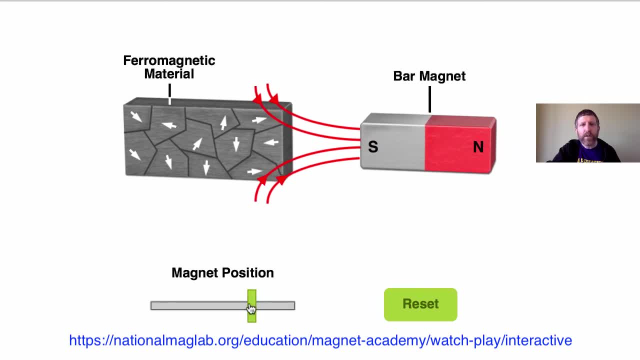 Watch what happens to the alignment of those domains. when I bring this close, Notice that the domain that is aligned with it is actually bigger. The domains that are not aligned get smaller, But what you end up with is the same thing in either situation: All these domains. 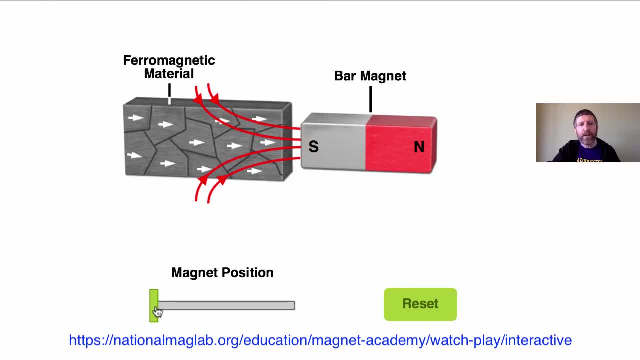 are aligning with this external magnetic field And when I, even when I pull away the permanent magnet, those domains stay aligned. So now what I have is I have the field. Now this field is going to have right here. this thing is now a new permanent magnet. Now, if I shake or heat, 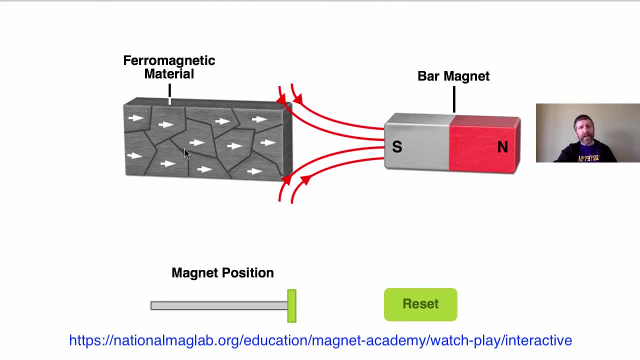 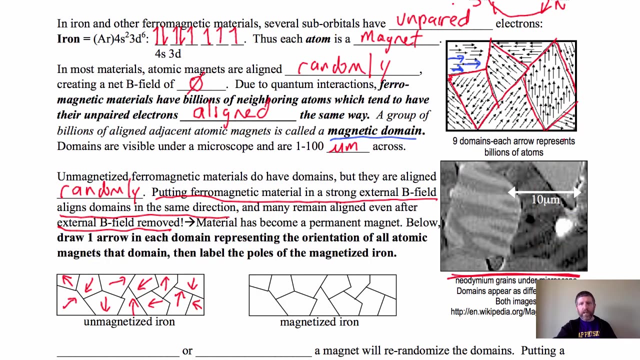 this ferromagnetic material, or slam it really on the ground, or heat it to what is called the Curie temperature. those get re-randomized and it goes back to that. So that is how you make and then break a permanent magnet. So here's our magnetized iron, if they are all lined up, and they're never lined up.